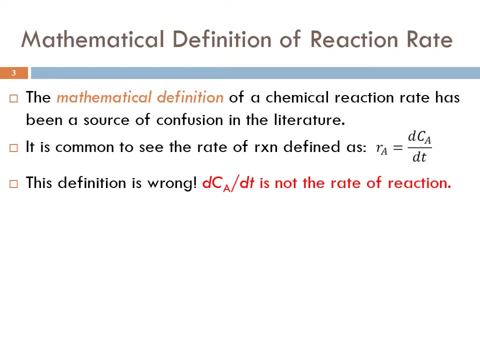 This definition is wrong. DCA by DT is not the rate of reaction. This is not the mathematical definition of the rate of reaction. The above equation is simply the mole balance for a constant volume batch reactor. It's a mole balance. This is a result of a mole balance. 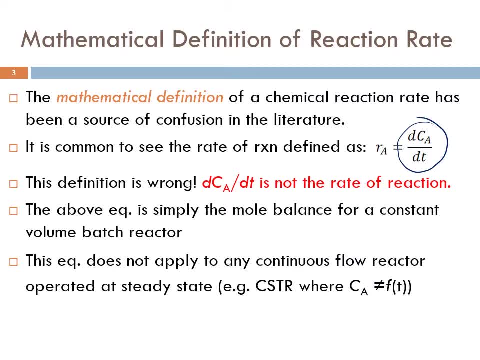 This equation does not apply to any continuous flow reactors operated at a steady state, For example, the CSTR that we're going to talk about here For the CSTR, For the CSTR. In the CSTR, the concentration is not a function of time. 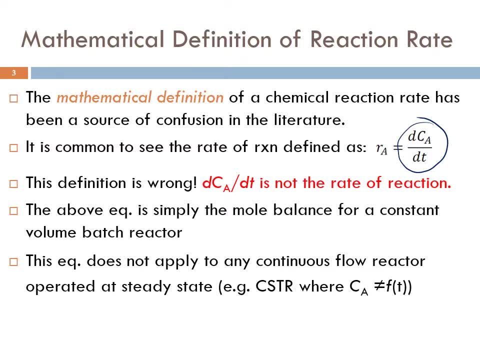 So DCA by DT is 0.. Does that mean you don't have a reaction in this type of reactor? No, that's not correct. So this is not the mathematical definition of the reaction rate. This is only a mole balance for a constant volume batch reactor. 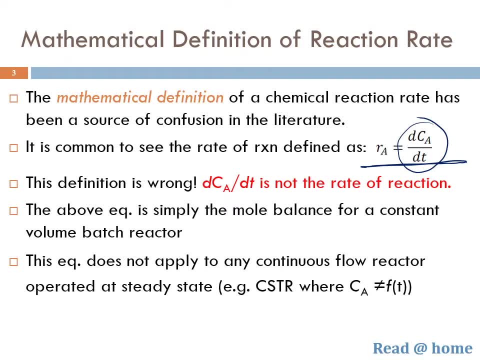 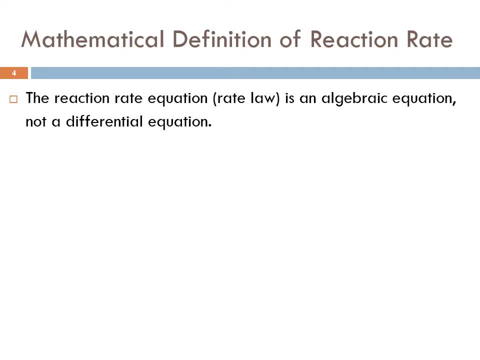 There are some slides that you might want to read at home. What is then the mathematical definition of a reaction rate? the reaction rate, the reaction rate equation, or known as the rate law, is an algebraic equation, not a differential equation. for example, for A goes to B, the 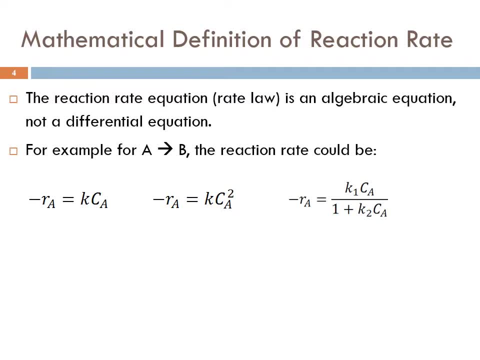 reaction rate could be: minus r equals k times C A, first order or second order. minus r equals k times C A to the power 2. or it could be in the form of the Langmuir-Henshelwood mechanism rate law. okay, so all of these are algebraic equation. these are the 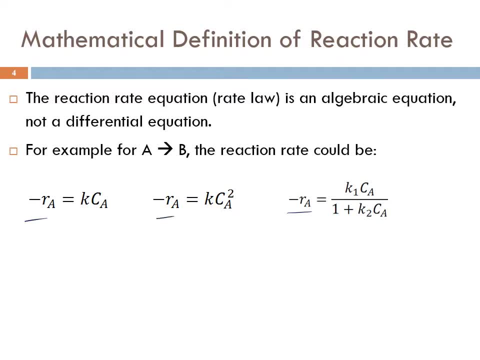 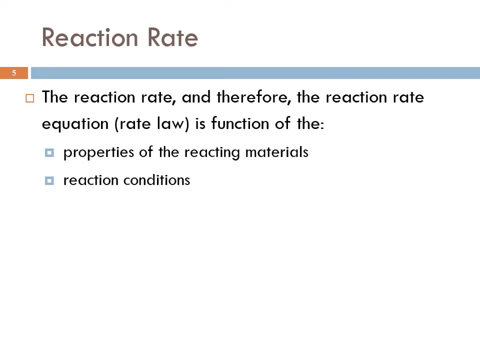 mathematical definition of this rate law, the reaction rate and therefore the reaction rate equation or the rate law, is function of the properties of the reacting materials, right? so when we say, for instance, C O reacts with O2, but I say dull, half O2 gives you CO2. and we know also, H2 plus half O2 gives you H2O, correct so? 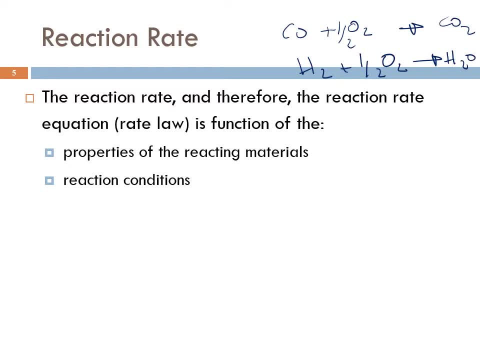 they look similar, they're all oxidation reaction, but they have different rates at the same condition. even if I use the same condition, the same everything, still the rate would be different for these two reactions because the properties of the reacting material is different in this reaction compared to this reaction. 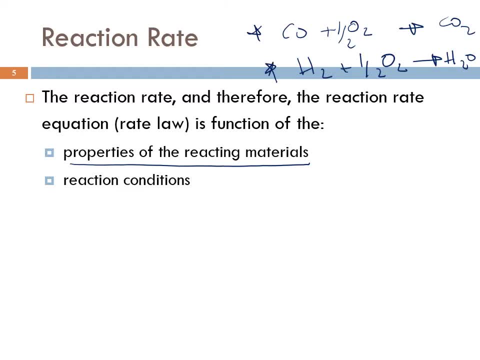 and also the reaction rate. and the reaction rate equation is function of the reaction condition. so let's take this equation. the rate of reaction of this equation is much higher at higher temperature, okay. it's much higher at higher concentration of reactant. it's much higher if I use catalyst, for instance, okay. so the reaction rate equation in 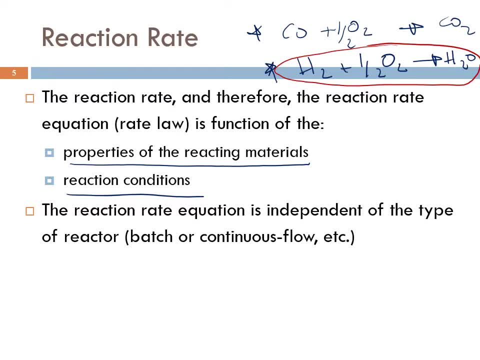 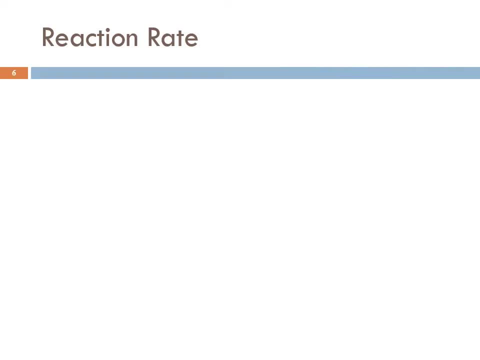 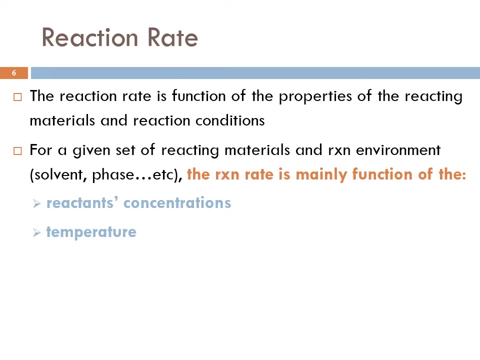 fact is independent of the type of reactor. it's not a function of the type of the reactor: batch or continuous load or anything else. the reaction rate is function of the properties of the reacting material and reaction conditions, as we just said for a given set of reacting materials, and reaction environment, for example. 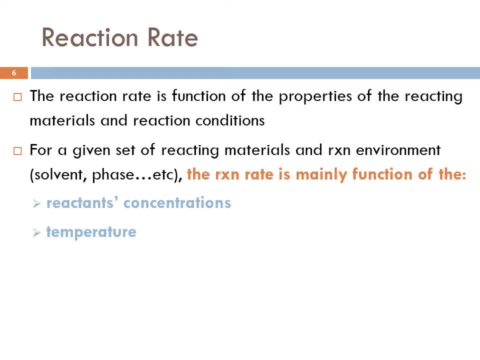 using a given solvent or running the reaction at a given phase. okay, that's what I mean for a given reaction environment and for a given set of reacting materials, for example CO and oxygen. the reaction rate is mainly function of the reactant's concentration, the temperature. so remember this: the rate of reaction is mainly function of 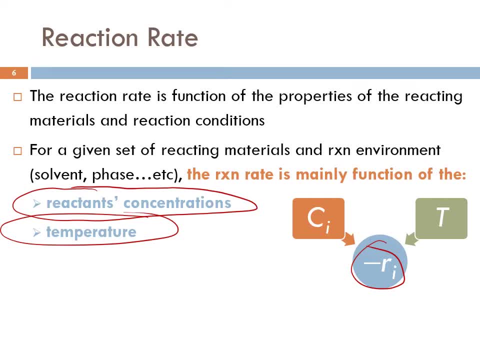 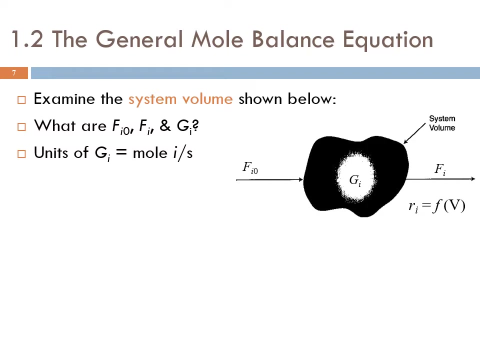 two things: the concentration and temperature. for catalyzed reactions, the reaction rate is also function of the catalyst activity, that's if I'm using a catalyst. so some catalyst gives you higher rate of reaction compared to others. but let's talk about that general mole balance equation, which is 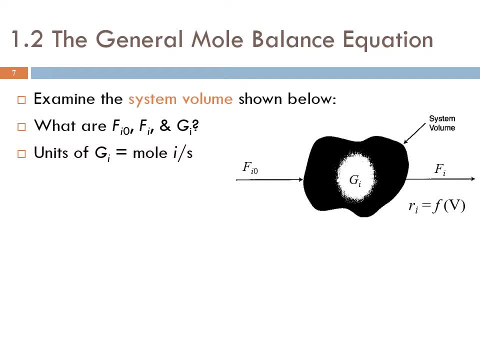 the most important or most topic in this chapter. that's the beef of this chapter, that's the title of this chapter and I'm sure that you like dealing with mole balance equations because you have studied it thoroughly in introduction to chemical engineering course. so let's examine this system volume or what's. 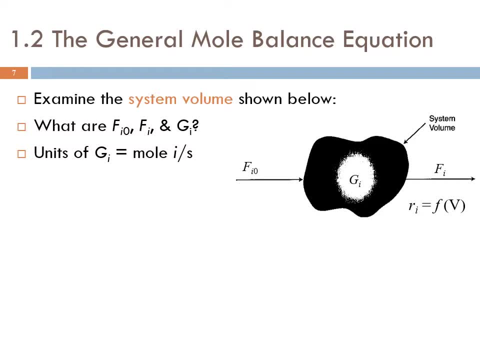 known as control, volume right, or just system. it's quite a system, okay. and the system of course has boundary right as a boundary. okay, that's sounds it okay. and then we have stream coming in and stream going out, type. let's discuss if I, what does if I. 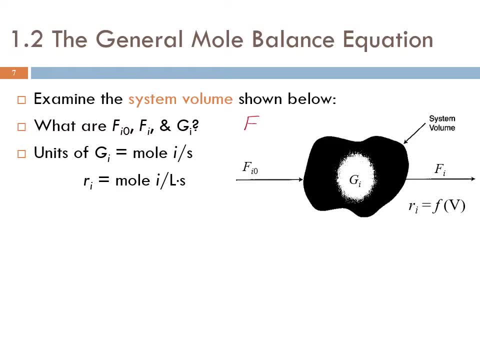 refers to. well, if in this course refers to flowrate flow rate, but in fact we care about molarged only. okay. we care about mauler Ph預, Maler flow rate- okay, because when you have reactions, then we care about burb waves, more furniture reacts, okay, and then we have an eye because this is the 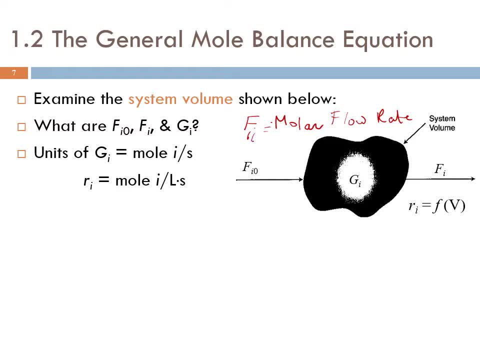 molar flow rate for species i and we have not. okay, that's a zero, referring to not okay. this is for the entering. this is the entering molar flow rate for species i. this is the exiting molar flow rate for species i. what is gi? well, gi is the generation rate. it's the generation rate for species i. that's. 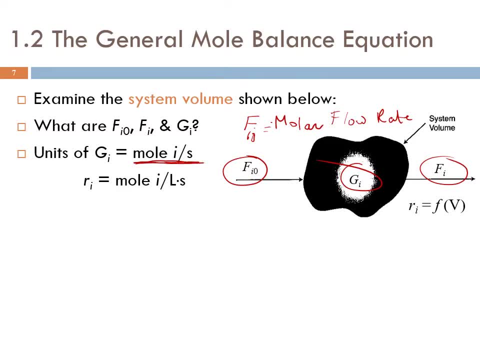 why it is mole i per second. come on, we say, well, now we have this much. five moles of a per second is generated in this system, inside this whole system. okay, that's gi. what about ri? well, ri is the rate of reaction, and we know that the rate of reaction has the units of mole i per liter. 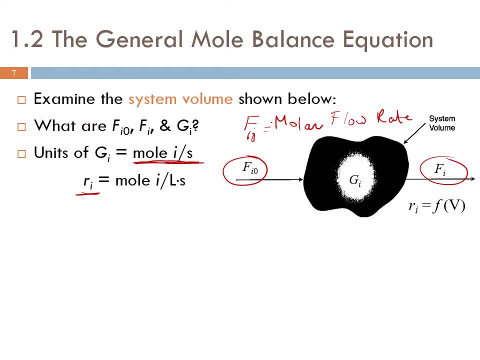 per second. right, you know that already, and here we're saying that ri is function of volume. by and by saying so, i mean it depends on in which volume of the reactor you are. are you, for instance, here, okay, or here, or here, or here or there or there, okay, that's what it means. 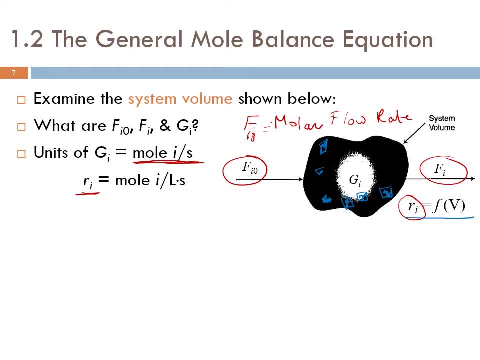 by the rate of fractions function of volume, and why the rate of fractions function of volume of volume. well, let's go to the basics. what is the rate of fractions function of its function of concentration and temperature? right, so maybe we don't have a mixer here? therefore, the concentration. 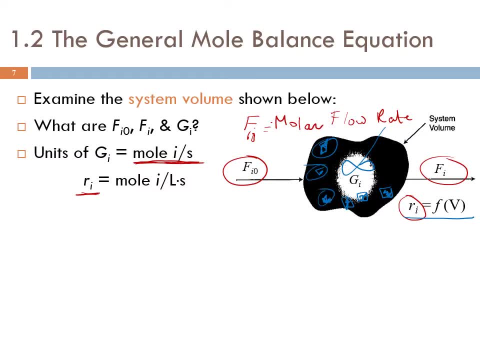 of i here is different than concentration of i here, and different concentration of i here. maybe the temperature here is different than the temperature here. so since these independent variables- the concentration of i and the temperature- are different at different locations, therefore the rate of fraction will be different at different. 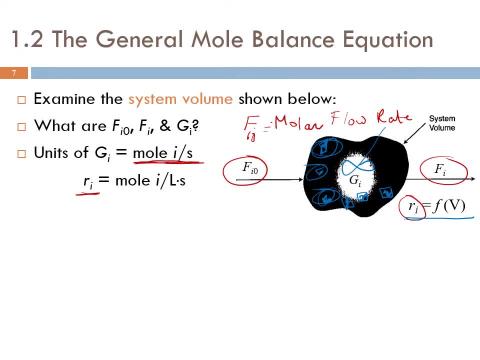 location. therefore the rate could be function of volume type. we explained that already. let's calculate gi from ri. let's calculate gi, the rate of generation, from the rate of reaction. can we do that? well, i'm sure you say, oh, that's really pretty easy, because ri has the units of mole i. 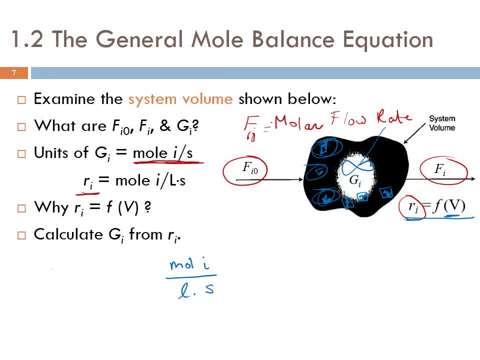 pair liter per second and you want mole, i pair second. you'll say: oh, then let's divide, multiply by the volume. so that's what you will say. let's multiply ri by the volume to get gi and the volume of this system, volume as in liter. so now the units are consistent. but the problem now is: 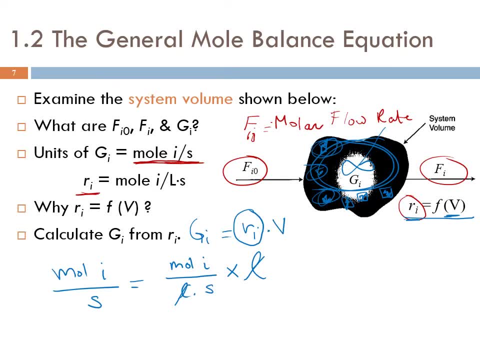 which r i you're going to take, because r i is different at different location, right? so which r are you gonna take? that's really confusing, right? well, it's not that. and confusing because you have dealt with similar situation when you took fluid mechanics. remember, if you have a fluid. 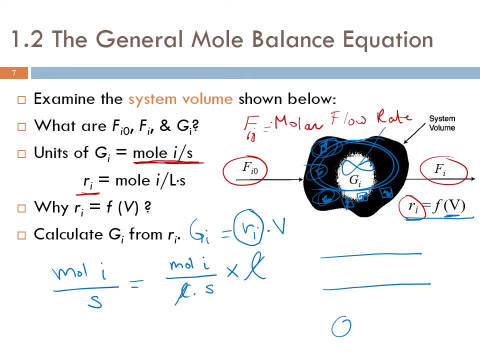 flow in a pipe and you have a turbulent flow. if you want the volumetric flow rate, for example cubic meter per second, right you would say: oh, let's look what the speed is, the velocity of the flow, and multiply it by that cross-sectional area- meter per second, this is meter square. however, the problem arises if you 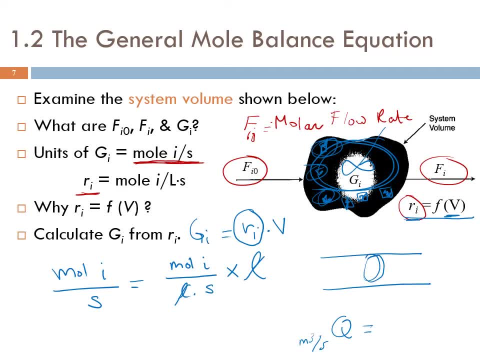 have. you have laminar flow and when you have laminar flow, the velocity at the middle is maximum right, and then it's zero at the boundary correct and maximum at the middle. so that's the velocity. so which velocity you're gonna take to multiply it by the cross-sectional area, which velocity you're gonna take? 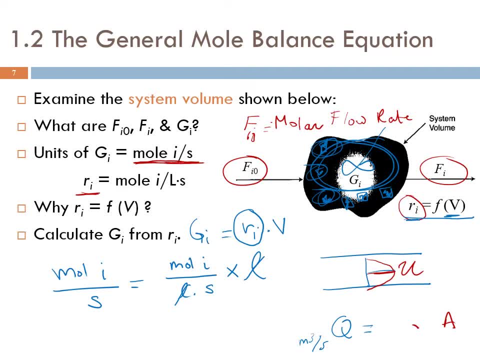 okay, so you can't take a single velocity here, but you're gonna integrate, correct. you're gonna integrate u times da from 0 to a for the whole cross-sectional area to get the total volumetric flow rate. so the same thing with the GI here, okay. 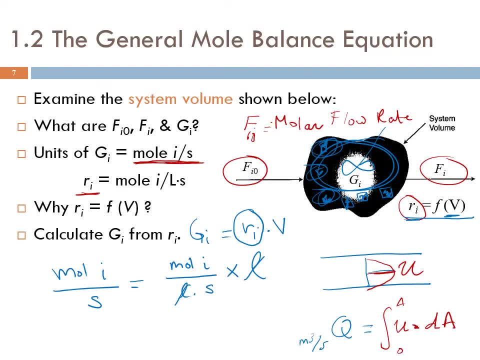 with the rate of, with a generation rate. so if you want GI, okay, you have to take RI and multiply by DV and integrate it from 0 to V, okay. in other words, what I'm doing is I'm taking this is small volume DV and multiplying it by the rate of reaction here and then take the next 6th volume differential. 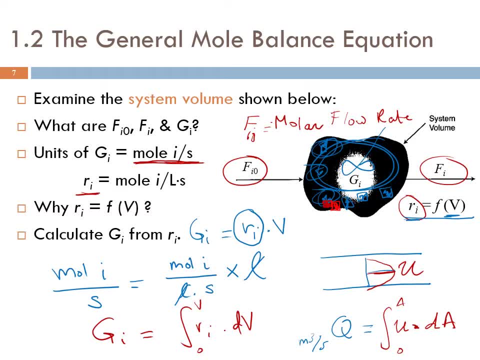 volume next to it and multiplying by that rate of reaction there, and then take the differential volume next to it, and that's differential volume, and multiply it by RI, right, and then take the next volume, and so on, right. so basically I am integrating a camel, integrating the whole thing, which is 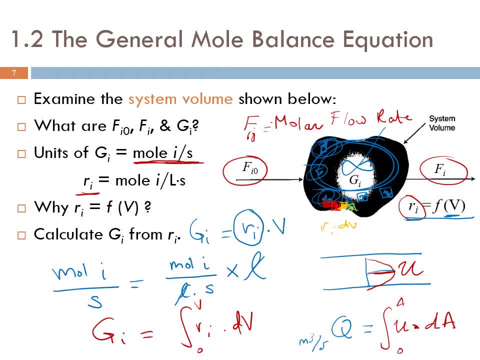 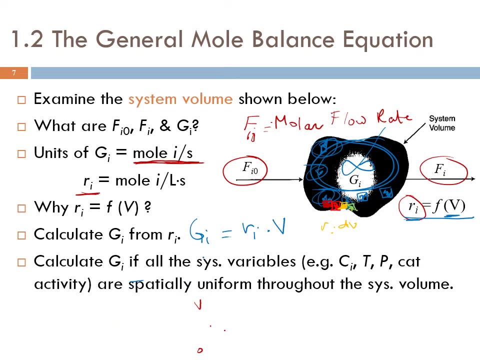 integration of RI DV. that's the definition of integration. okay, so it's a mess here. let me clean up. okay, so let's calculate, let's calculate GI, if all the system variables, example the concentration, the temperature, the pressure, the activity- are especially uniform, especially uniform throughout the system volume. so let's say that, let's. 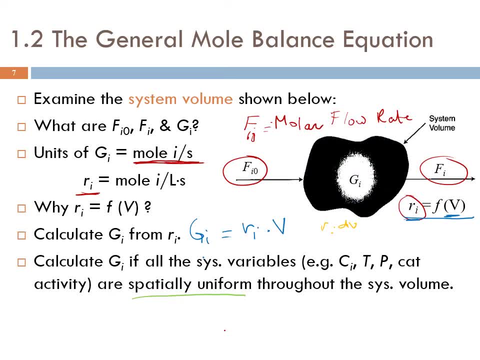 look any more important. let's look at concentration, and concentration are交价 temperature, the concentration of species I is the same everywhere. The temperature, the temperature inside the system is same everywhere. So if the concentration is the same everywhere, the temperature is the same everywhere. that means the. 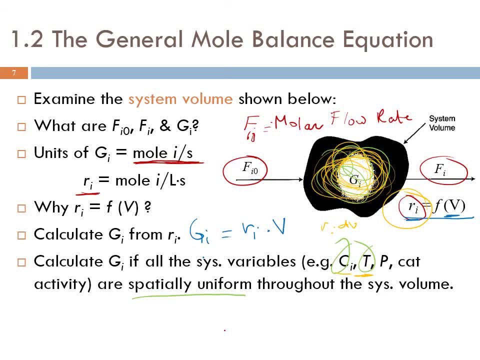 rate of reaction is the same everywhere, correct? So let's go to GI, GI: integration of Ri, dV from 0 to V. So now you will say, voila, Ri is not function of volume, Ri is really not function of volume. and when it's not function of volume, what happens? It goes outside. 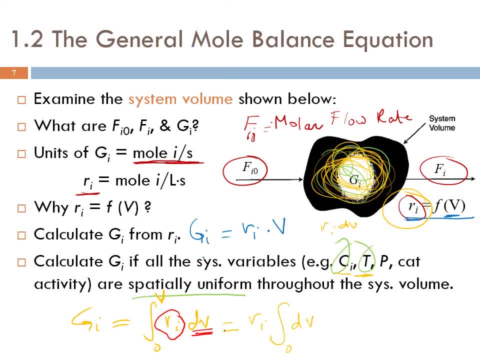 the integration right. We have integration of dV from 0 to V, and that is Ri. integration of dV is V from 0 to V, so that's Ri, dV, IV. and now it is correct. this equation, which we expected in the beginning, is correct only. 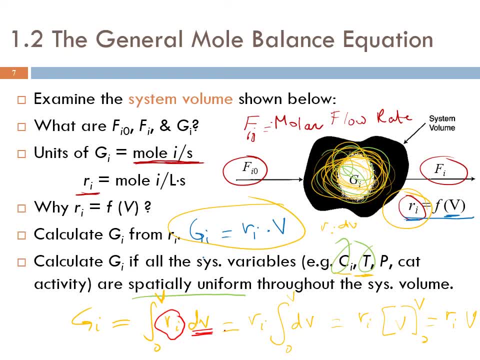 if the rate of reaction was not function of volume, meaning only if the concentration and temperature was the same throughout the system. okay, so here we go. we said FRI, FRI, yep, okay, so FRI is not function of volume. then basically, gi equals ri times g. 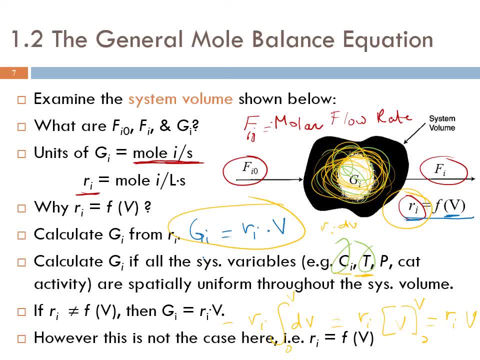 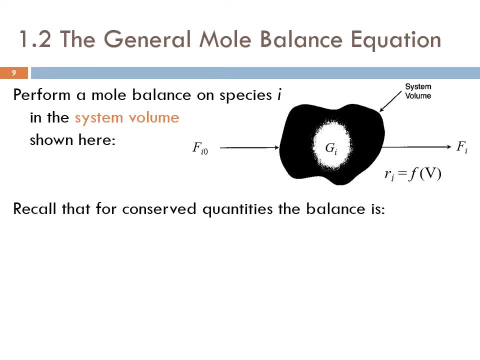 okay. however, this is not the case here. I mean the rate of reaction is function of volume. okay, so perform a mole balance on species i in the system volume shown here. let's perform a mole balance. recall that for conserved quantities. for conserved quantities, what does conserved quantity means? that means quantities that cannot be created. 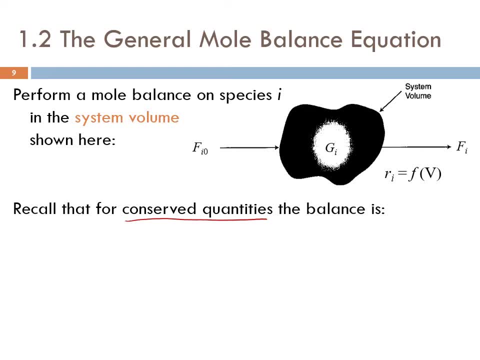 stated know all destroyed, right. it cannot be created means cannot be generated from nowhere. and it can be destroyed mean cannot be consumed to nothing. okay, for conserved quantities we have accumulation equal input minus output, right, that's the balance for a conserved quantity. what are conserved quantities? for example, mass? mass is conserved in classical. 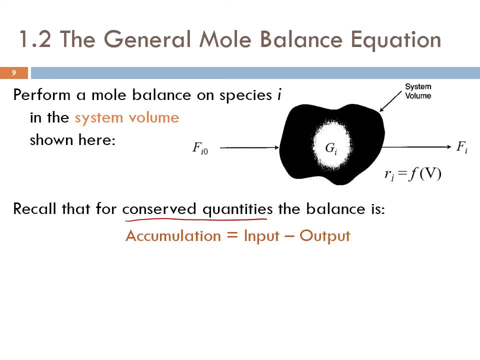 chemical reactions, right energy is conserved, right momentum is conserved, all these quantities are conserved. So when we balance it, we say accumulation equal input minus output. However, for non-conserved quantities, meaning for quantities which can be created or quantities which could be destroyed, the balance becomes accumulation equal input minus. 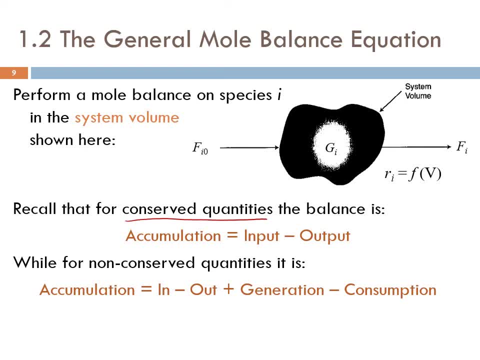 output plus generation, minus consumption. An example again for that would be this reaction: H2 plus half O2 gives you water right Through this reaction. well, I have here one and a half mole of reactant entering. If the reaction proceeds to the end, you have one mole only. 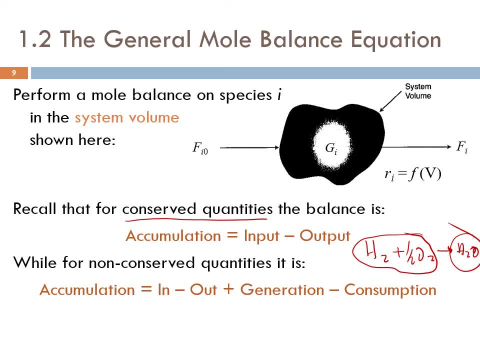 So what happened to that half mole? It got destroyed, It got consumed, right? If you look at hydrogen, here we have one mole of hydrogen, Here you don't have any mole of hydrogen, right? You say, no, I have H2 here. No, no, 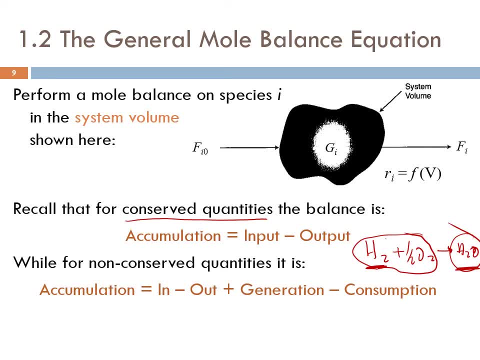 This is H2O. It's a different species. So we don't have a molecule H2 here. So we have H2, one mole of H2. at the beginning, at the end of the reaction, after completion, We don't have hydrogen. We don't have one mole of hydrogen. What happened to that mole of? 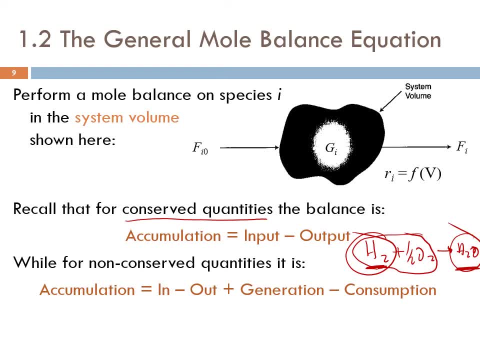 hydrogen, It got destroyed. Same thing I generated one mole of H2O. So number of moles is not conserved, It's not a conserved quantity. Therefore, if I want to balance it, I say accumulation. Accumulation equals input minus output, plus generation, because it can be created minus 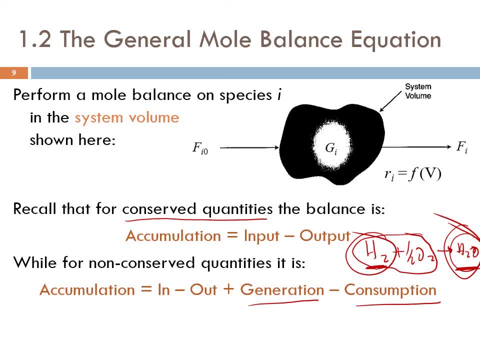 consumption because it can be destroyed. Or some people or some textbook will sum up these two and call it generation or production. So basically the generation means generation minus consumption. So let's see: Input minus output. plus generation equals accumulation. So what's the input to the system? 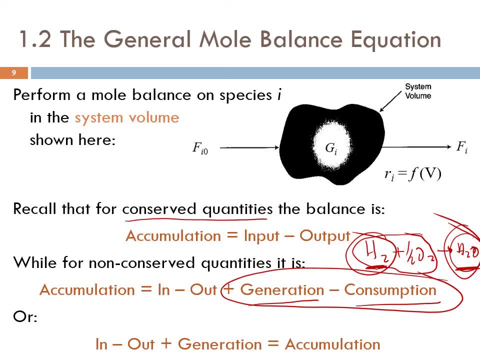 Well, basically the input to the system for a species I. So I'm doing a mole balance on a species I around this system, around this system. So when I say input, input to the system for these number of moles of the species I, So that is FI0.. That's the input. 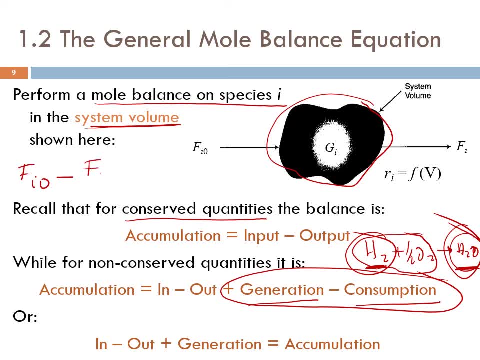 Minus output Output is FI correct. That's the output, That's the input. this upper plus generation, that is gi. and see that they all have the same units. if i not is mole per second. if i is mole per second, gi is mole per second right and it equals accumulation. 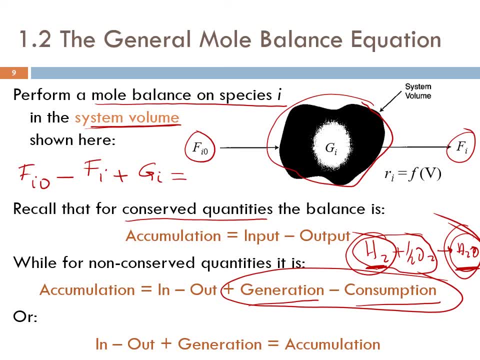 accumulation. accumulation of what of moles? right. number of moles in i. so an accumulation is calculated by d and i by dt, right. that's the rate at which the number of moles is accumulated within that system and also has a unit of mole per second. okay, so that's the balance for the system, okay, what? 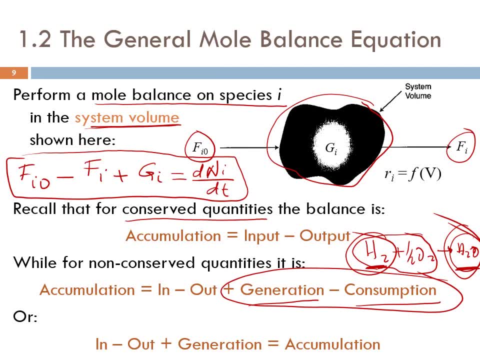 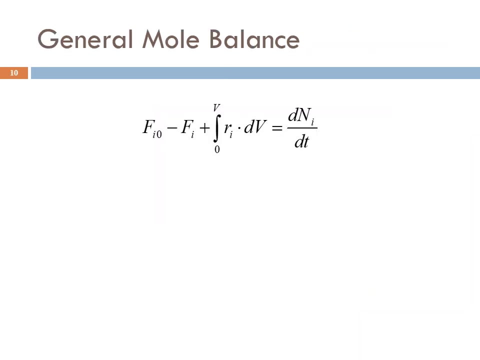 does gi equal? what does gi equal? well, let's rewrite that above equation, let's write it here. so that is, if i not minus, i plus gi, what does gi equal? well, gi equals the integration of ri dv from zero to v, equals accumulation, which is d and i by dt. so now i have a general mole balance.